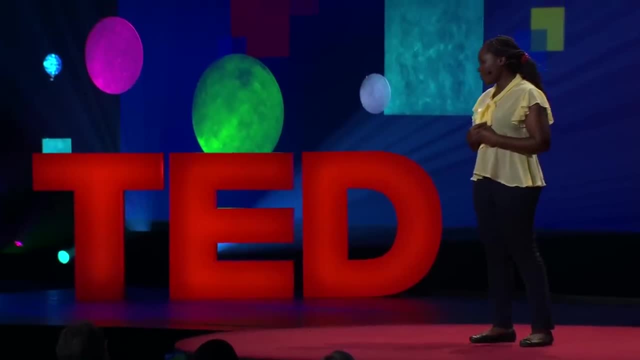 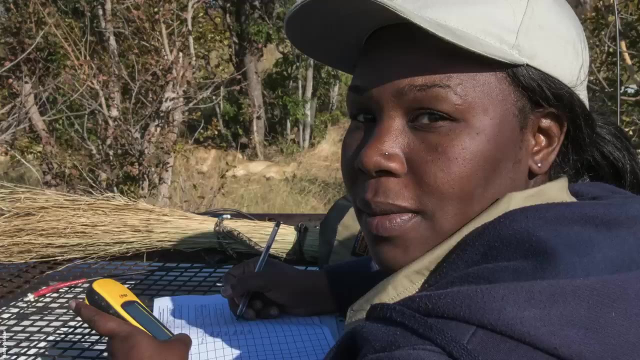 Because they don't meet a lot of conservationists who look like me. When I was growing up, I didn't even know that wildlife conservation was a career. The first time that I saw a wild animal in my home country was when I was 25 years old. 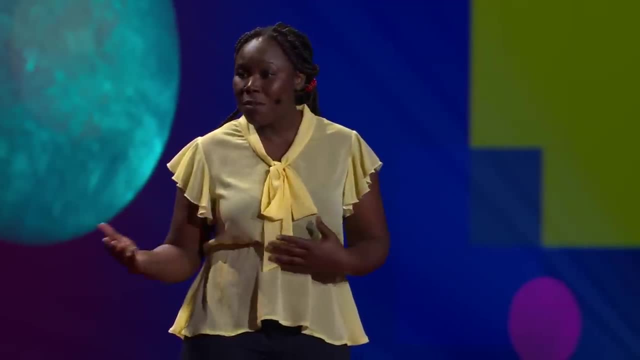 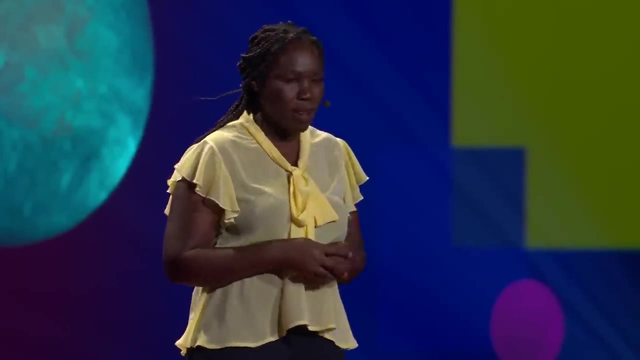 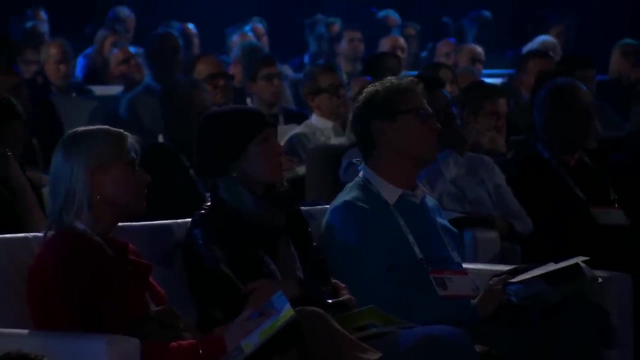 Even though lions and African lions lived just a few miles away from my home. This is quite common in Zimbabwe, as many people are not exposed to wildlife, even though it's part of our heritage. When I was growing up, I didn't even know that lions lived in my backyard. 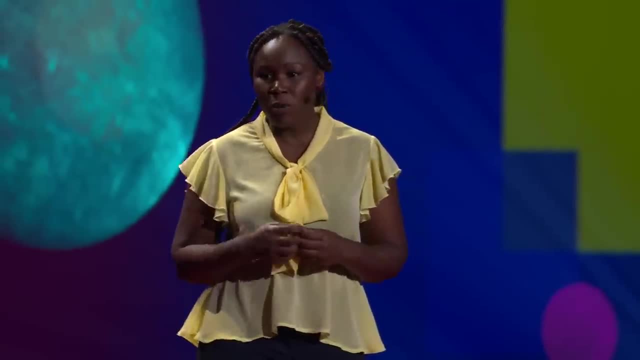 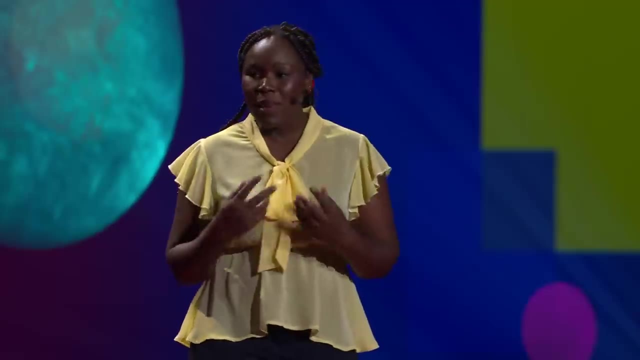 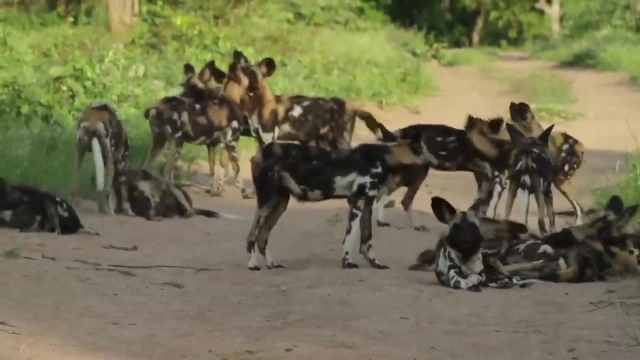 When I stepped into Savé Valley Conservancy on a cold winter morning 10 years ago to study African wild dogs for my master's research project, I was mesmerized by the beauty and the tranquility that surrounded me. I felt like I had found my passion and my purpose in life. 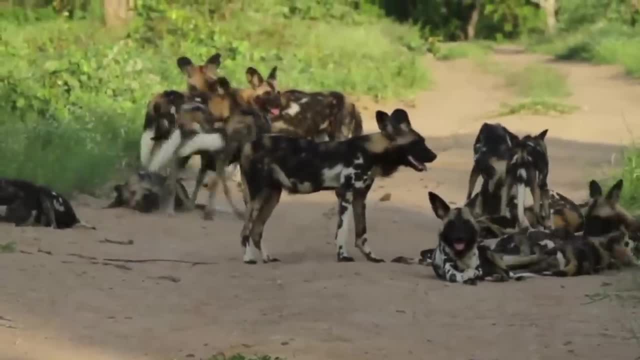 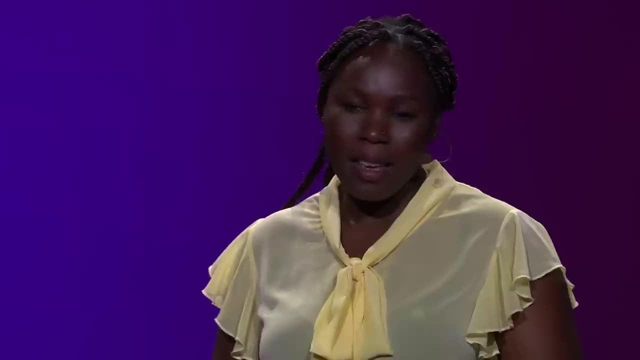 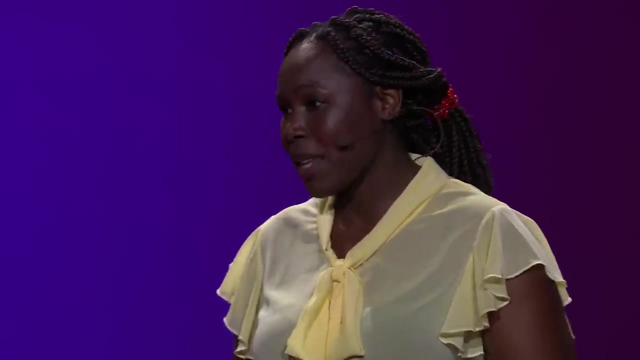 I made a commitment that day that I was going to dedicate my life to protecting animals. I think of my childhood school days in Zimbabwe and the other kids I was in school with. Perhaps if we had a chance to interact with wildlife, more of my classmates would be working alongside me now. 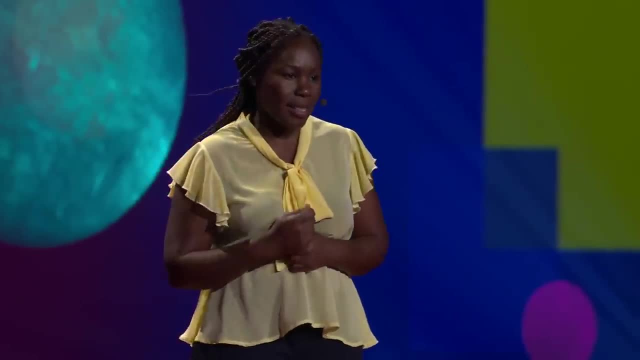 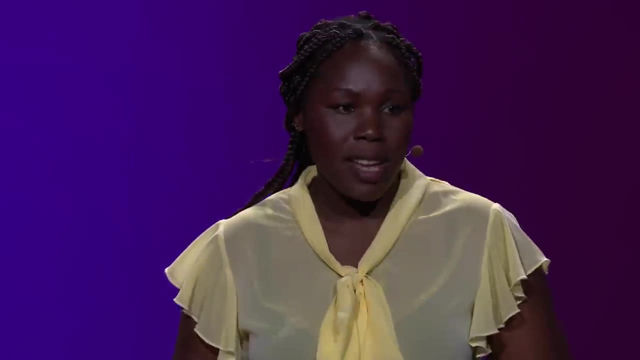 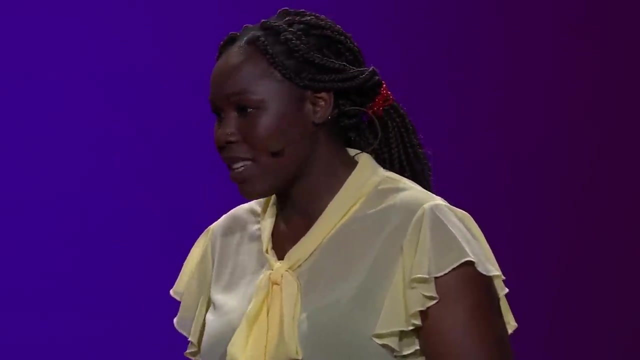 Unless the local communities want to protect and co-exist with wildlife, all conservation efforts might be in vain. These are the communities that live with the wild animals in the same ecosystem and bear the cost of doing so If they don't have a direct connection or benefit from the animals. 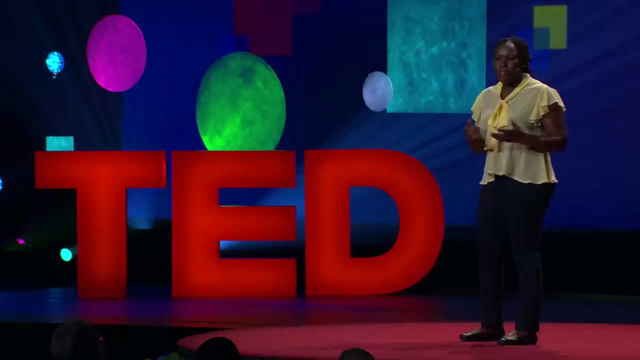 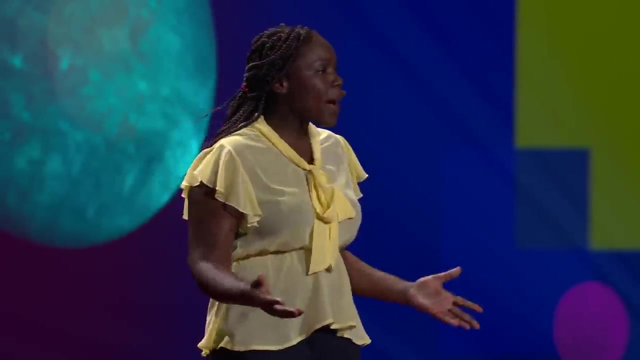 they have no reason to want to protect them. And if local communities don't protect their wildlife, no amount of outside intervention will work. So what needs to be done? Conservationists must prioritize environmental education and help expand the community's skills to conserve their wildlife. 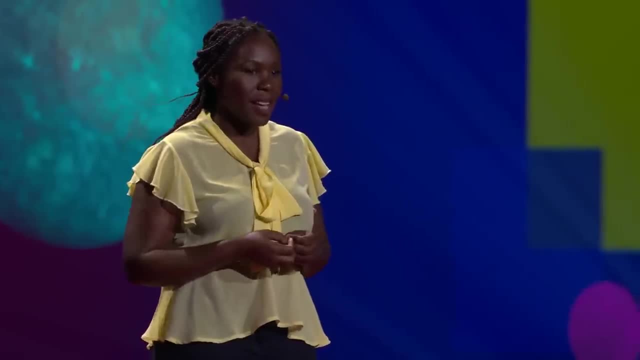 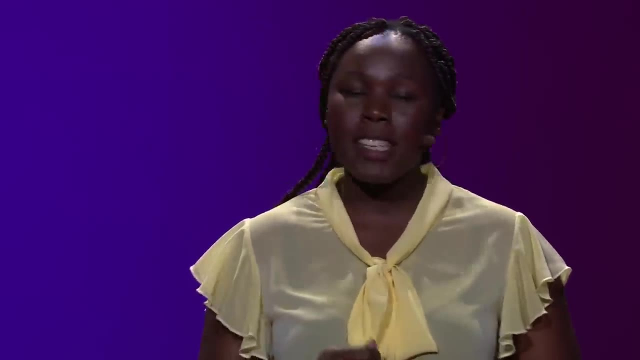 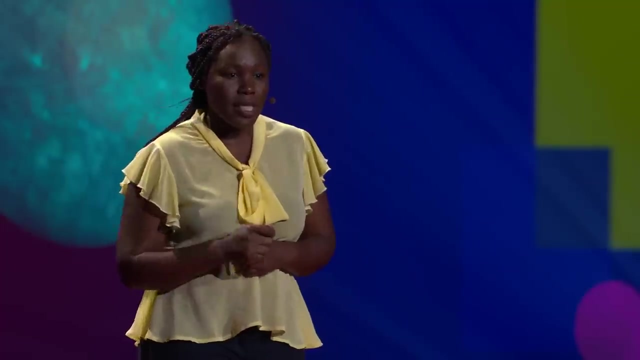 Schoolchildren and communities must be taken to national parks so they get a chance to connect with the wildlife. At every effort and every level, conservation must include the economies of the people who share their land with the wild animals. It is also critical that local conservationists 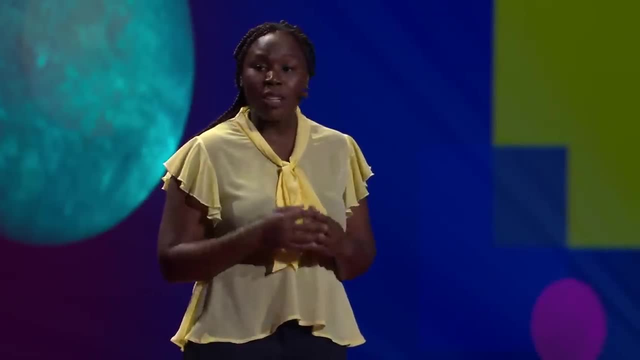 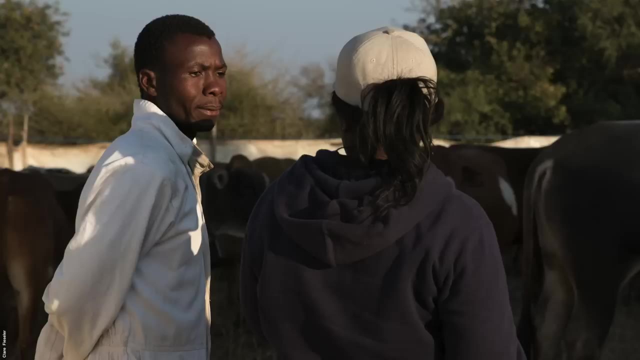 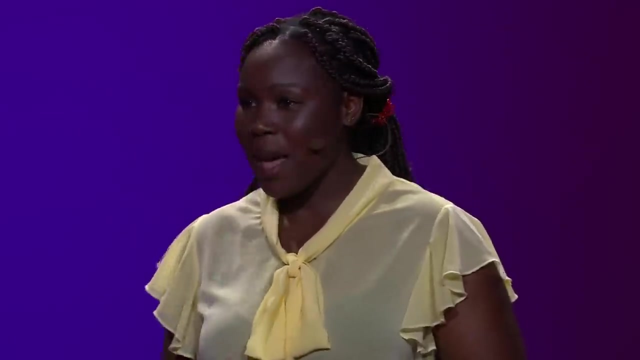 be part of every conservation effort If we are to build trust and really embed conservation into communities. as local conservationists, we face many hurdles, from outright discrimination to barriers because of cultural norms, But I will not give up my efforts to bring indigenous communities.